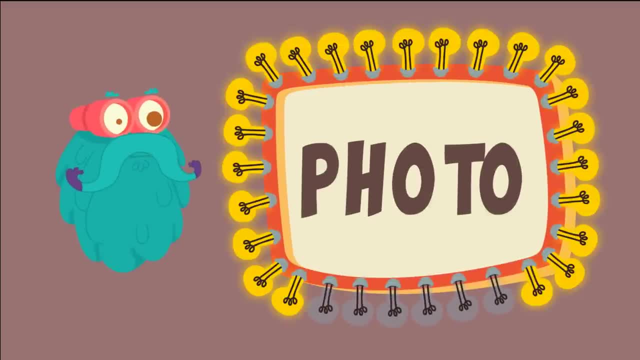 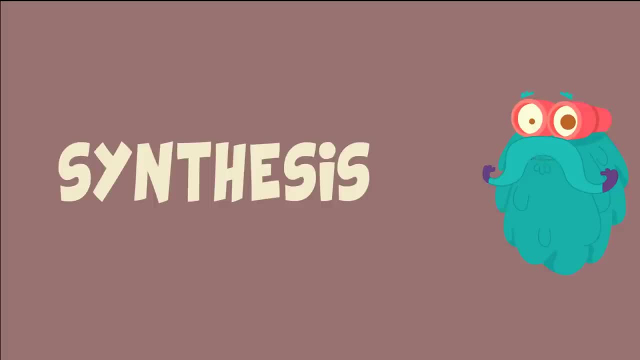 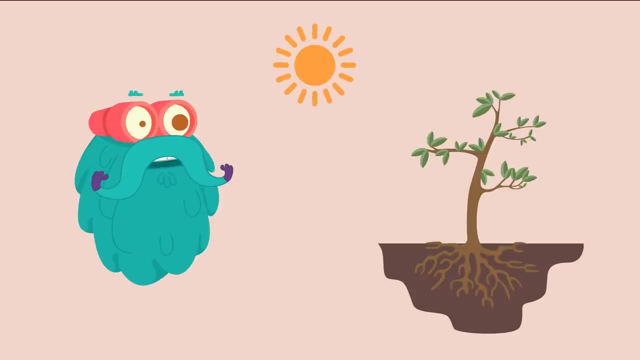 I'll tell you what it means. Photo is a Greek word for light and synthesis is a Greek word for putting together. Now it's simple: Photosynthesis is using light to put things together. Plants use this process to make their food with the help of sunlight, water and carbon dioxide. 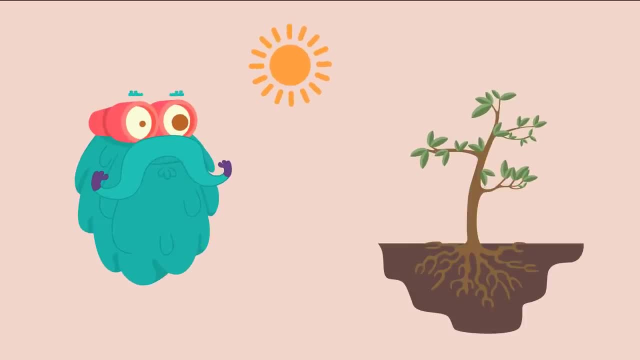 Did you know that plants breathe just like us? You didn't. Well, now you do. Plants have tiny openings, called the stomata, present in their leaves, through which they take in carbon dioxide. Yes, they breathe in carbon dioxide and give out oxygen. 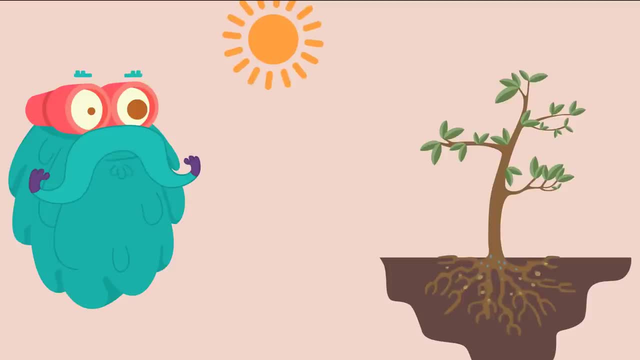 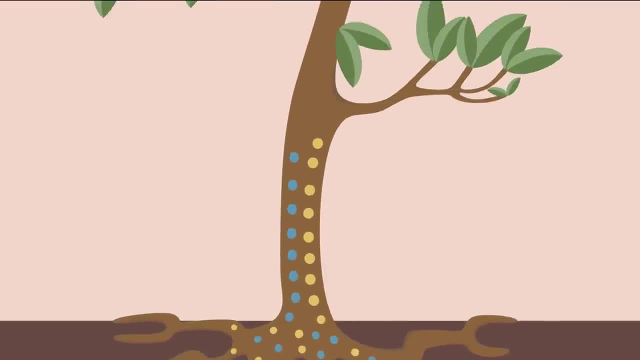 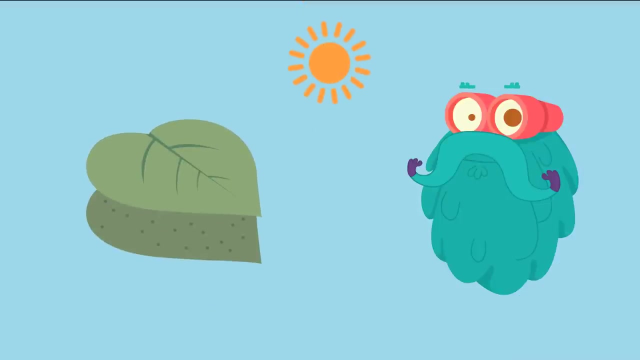 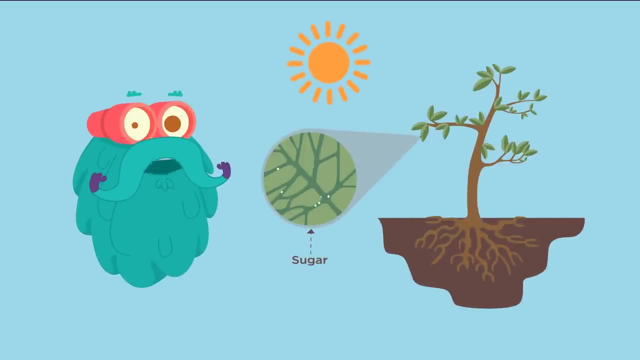 They also use water and other nutrients to make food which is absorbed by their roots. The leaves contain tiny pigments called the chloroplasts. These pigments take in carbon dioxide, Water and sunlight and turn them into sugar and oxygen. The sugar is then used by the plants as their food and the oxygen is given out into the atmosphere. 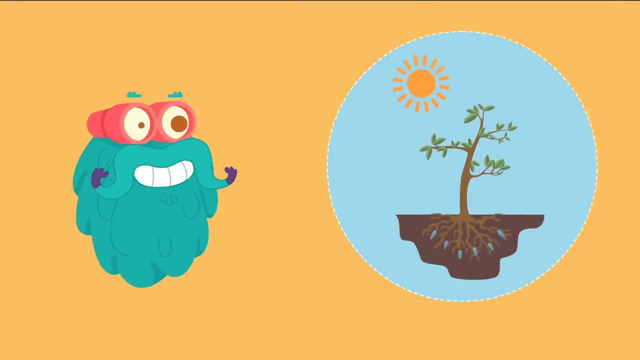 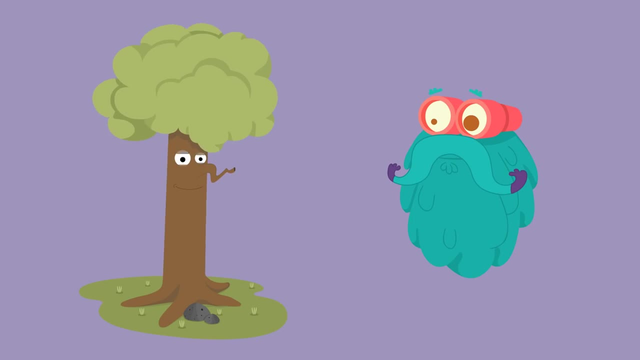 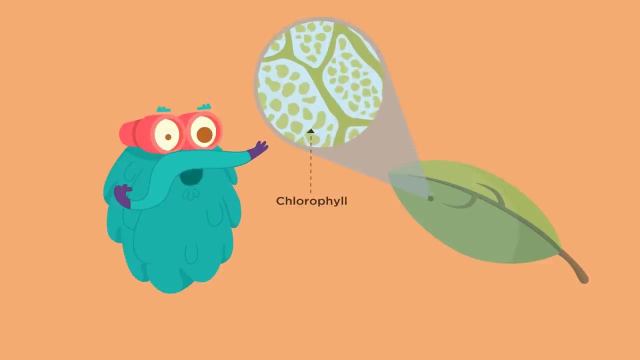 This process as a whole is called photosynthesis. Am I right, Mr Tree? Yes, you are Trivia Time. Chlorophyll is a green pigment that is found in the chloroplast of the plant. It makes the plant look green. 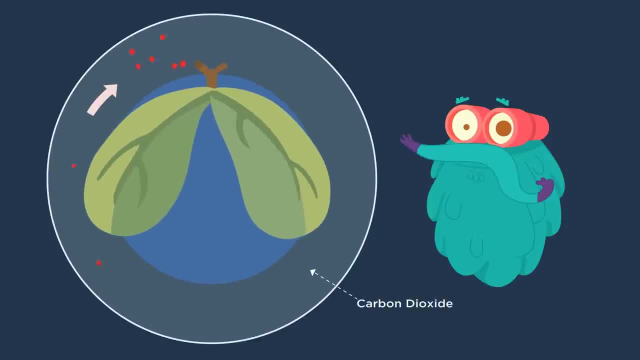 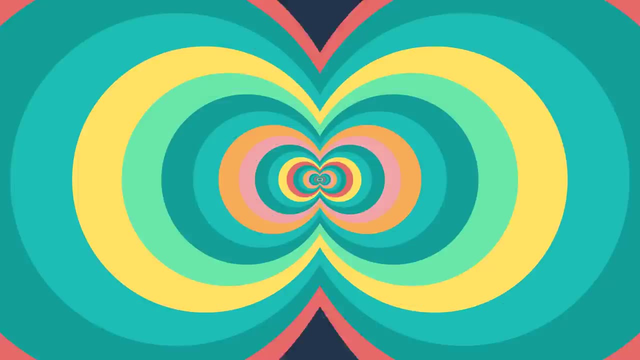 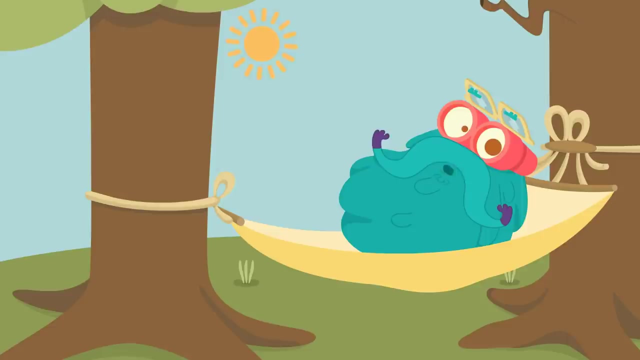 Plants are often known as lungs of the world, as they take in carbon dioxide and give out oxygen which the humans breathe. It's time for some more sunbath. So this is me zooming out. Tune in next time for some more fun facts.